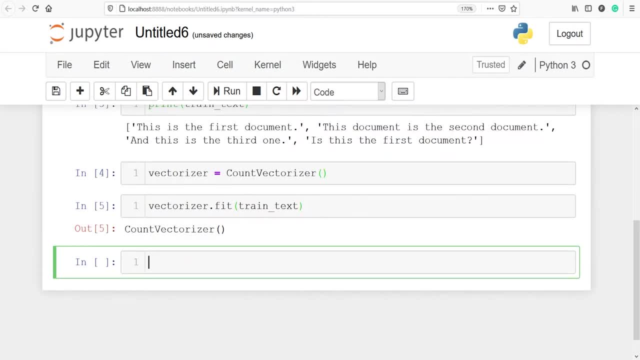 text. Let's execute our code. The fit function will pre-process all of the sentences we pass in. It will convert all these words into lowercase And generate a token of words. Let's get the feature names the count vectorizer has extracted from your text. Let's call this vectorizer and from this we will call the property get feature names. 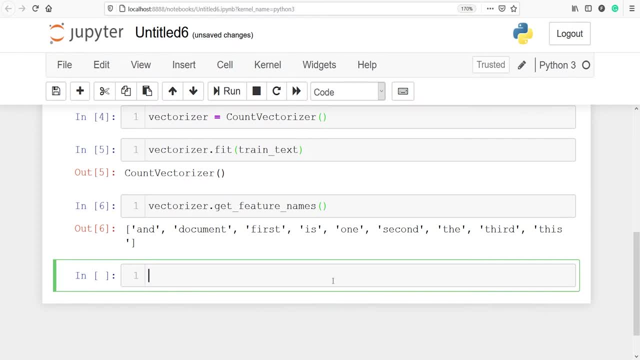 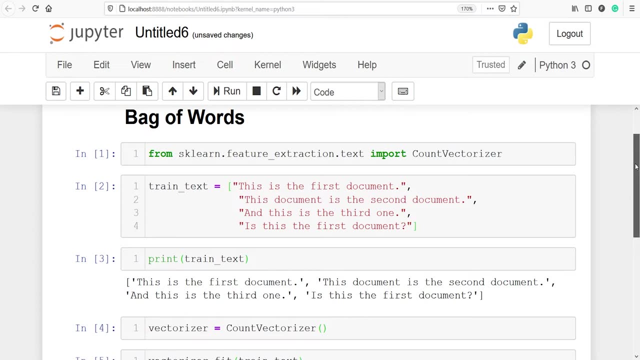 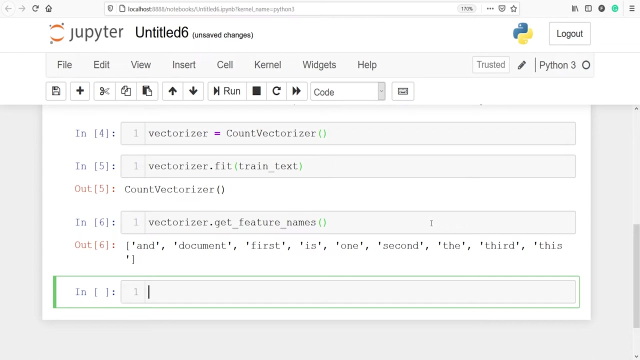 You can see that all the words have been lowercased and these are the feature names which have been extracted from the four sentences present in this variable train underscore. The vocabulary property on the vectorizer object will give you all of the words that the vectorizer can present. I'll call our object vectorizer. 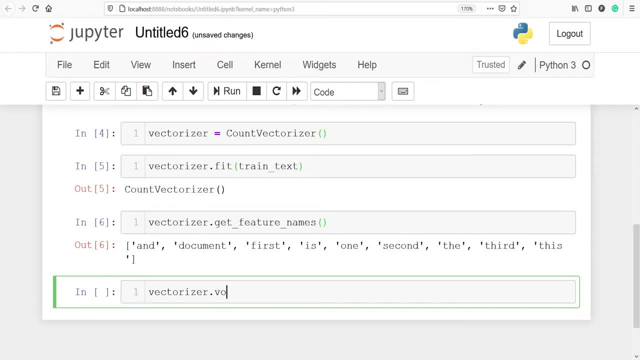 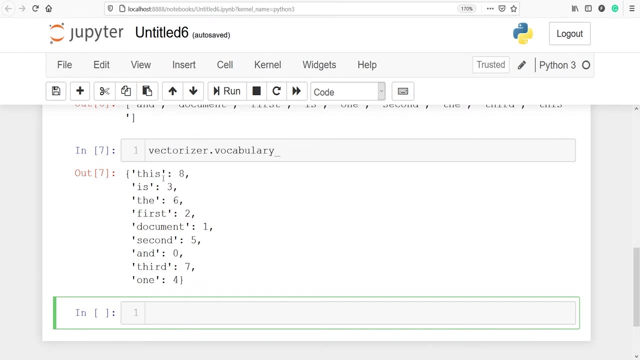 and then I will call the property vocabulary. Let's execute our code. In the output you can see we got the vocabularies and these are the associated unique ids, Since there are total nine vocabularies: one, two, three, five. 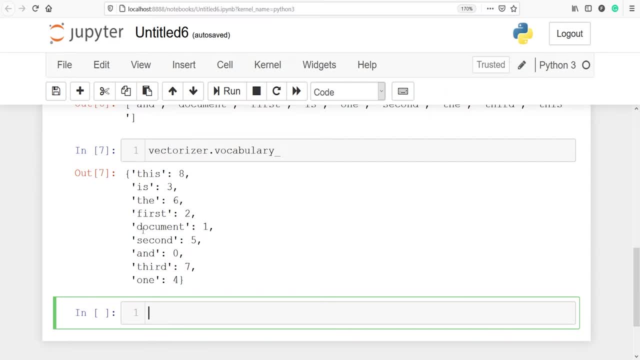 Attend all seven items to initialize the main petiz: three, four, five, six, seven, eight and nine. We got the nine unique numbers, starting from zero, ending at eight. The vocabulary here is a dictionary that maps every word in your input text on which the vectorizer has been trained to a unique integer ID. This numeric 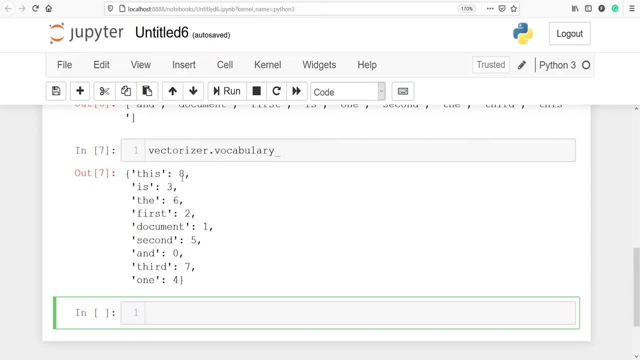 ID is used to represent a particular word in your text. You can use the get function on the vectorizer to access the numeric ID associated with a particular word. For example, we want to get the numeric ID of the word document. we can get it. I'll call the object. 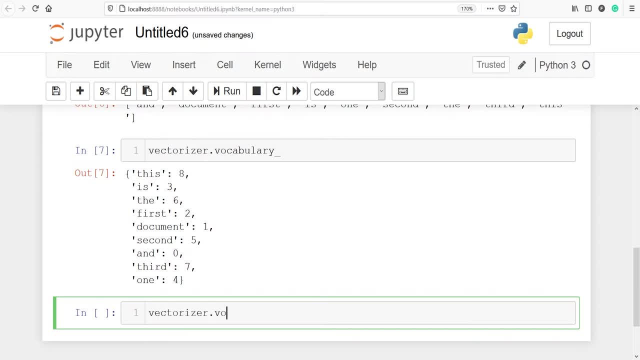 vectorizer and then I will call vocabulary underscore, then I will call the property get and I want to get the numeric ID of the word document. I'll copy this code from here. I'll copy this word from here, Paste it here. Let's execute our code and you can see we got the numeric ID of our word. 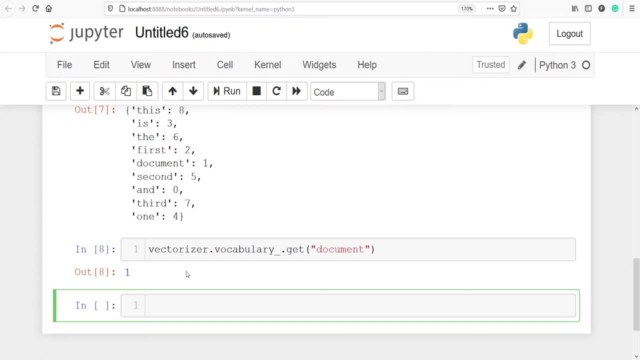 document. and here also it is one. here also it is one. Next, we will convert our sentences saved in the variable train underscore text into bag of words representation: by calling the transform function of the count vectorizer. I'll make one variable transform underscore vector. Now I will call the object vectorizer. From this I will call the property transform. 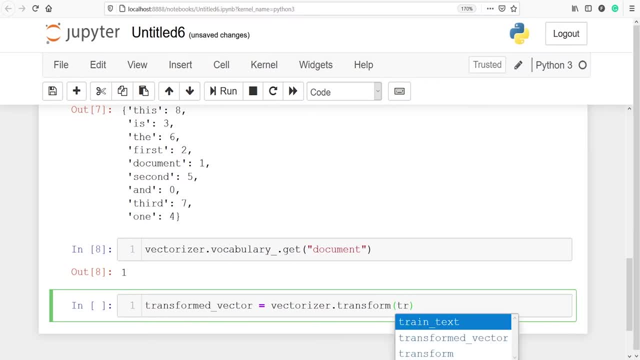 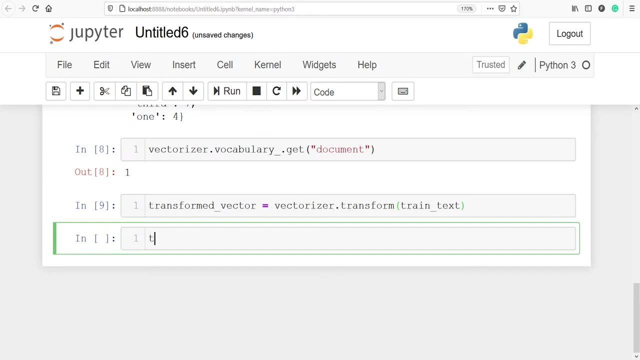 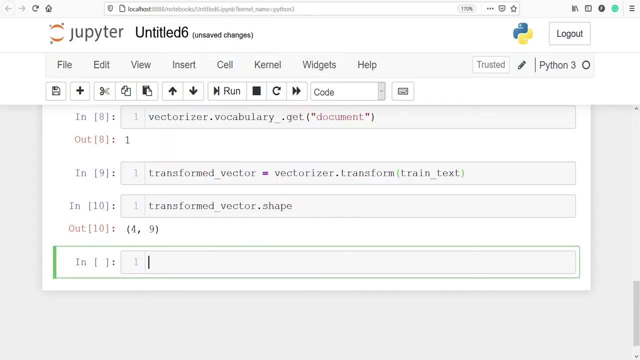 and I'll pass our variable train underscore text. Let's execute our code. Let's check the shape of this variable: transformed vector dot shape. The result is a transform vector of numeric representation. shape of this vector is 4 by 9, because we are having four sentences and nine. 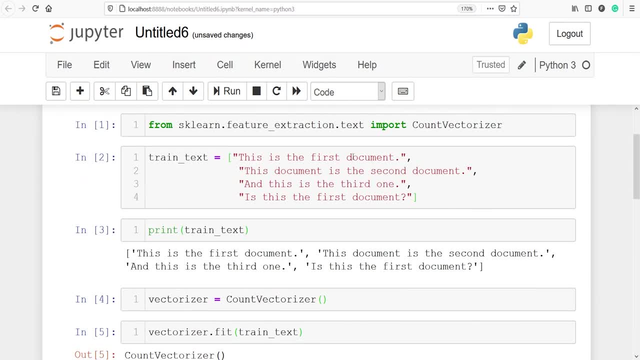 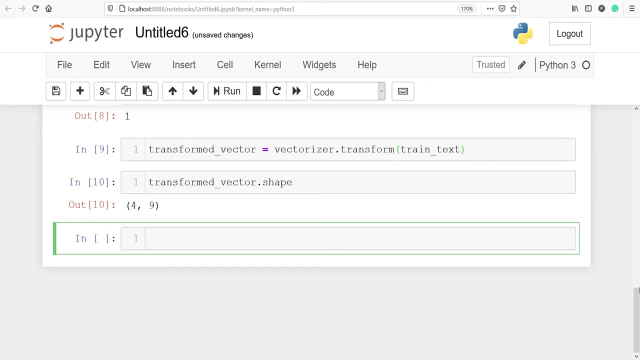 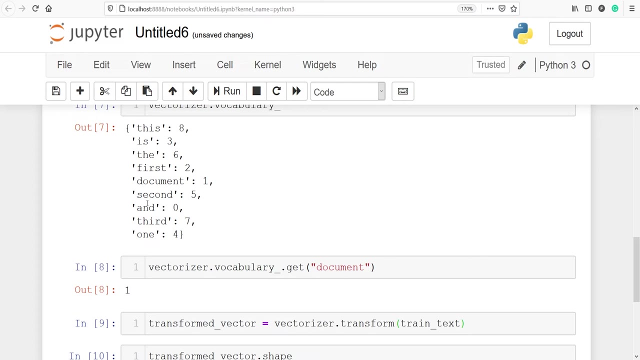 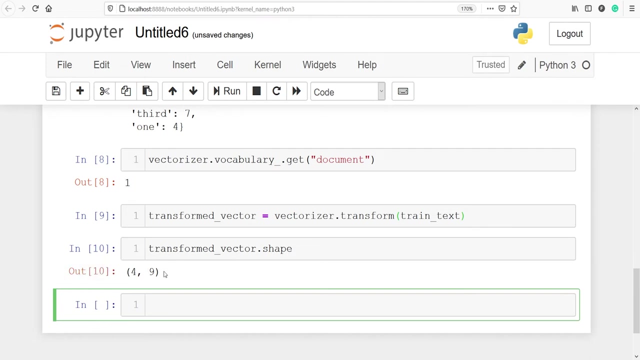 vocabulary. here you will see we have four sentences: 1, 2, 3 & 4. that's why we got four here and nine here, because we are having nine vocabulary. and this vocabulary are the features one, two, three, four, five, six, seven, eight and nine. so we got four by nine. you can also understand it as rows and columns. we 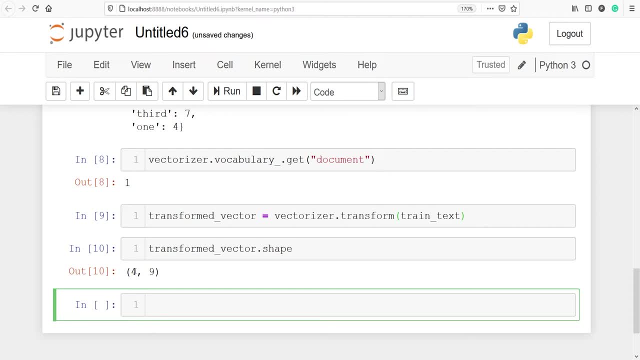 have four rows and nine columns, where rows are our sentences and columns are the vocabulary or the feature names. let's call to array function to see what the bag of representation looks like. I will call our variable transformed vector and then I will call to array. let's call to array. 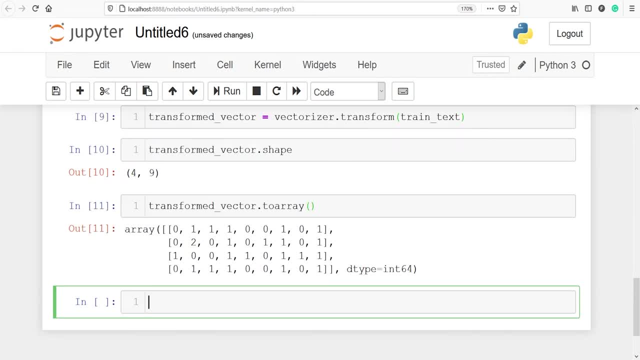 let's execute our code. the count vectorizer gives us a frequency based representation of words in our input text. and there are. these are the features here. these are the features here. a frequency of one is associated with every word in the sentence. if a word occurs twice, we will get two here, and if 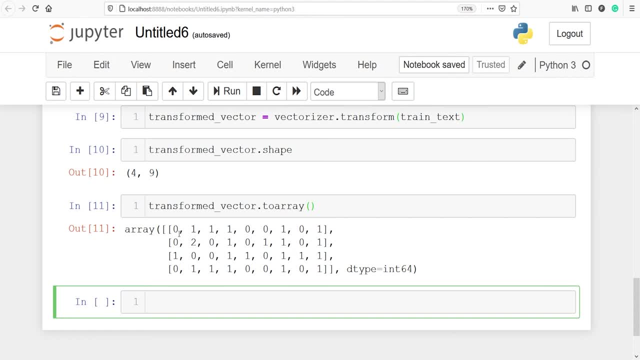 the word is not found, we will get zero here. let's test it on a new text. I'll. let's test it on a new text. I'll make one variable test, underscore text. I'll make a python list and I'll write a sentence. I am learning NLP. let's execute our code. let's print our variable test. 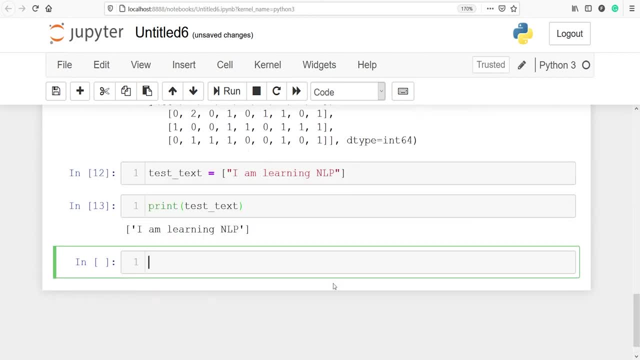 underscore text in the output you can see we have one sentence here. I am learning NLP. if these words are not found in the vocabulary of our count vectorizer, we will change it to: while count vectorizer. or we will change it to: I encounter that hereMP, for if these words are not found in the vocabulary of our count vectorizer, we will leave that as blank. 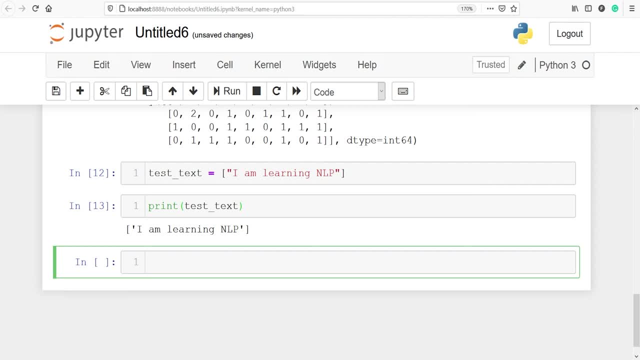 will get 0 at all places, because during fitting the count vector this sentence was not present. if any word is found in the vocabulary, we will get 1 or its frequency. Let's transform this. we will call our vectorizer object. then I will call the property transform. 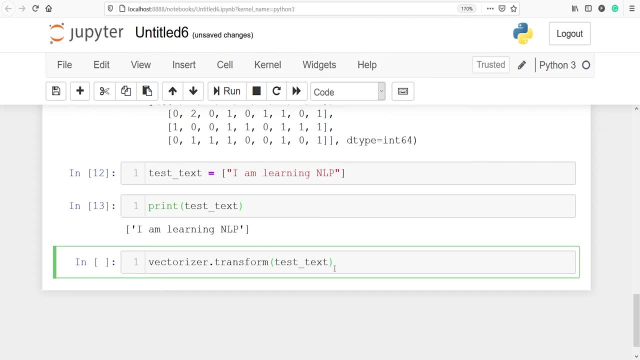 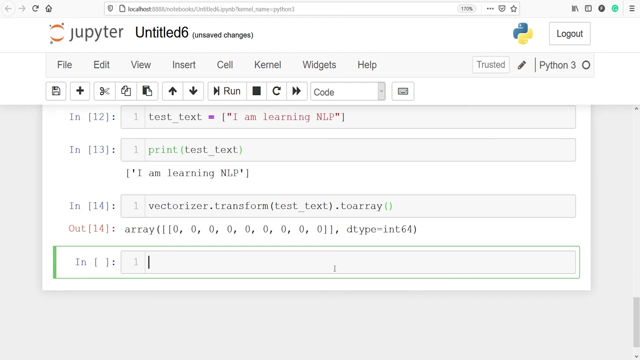 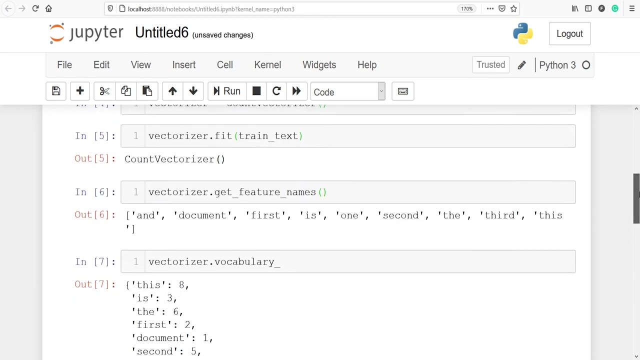 and I will pass our test, underscore text and convert it to true array. Let's execute our code and here we will see we got 0: 0 here. because let's look at the vocabulary or the feature names, both feature names and vocabulary are same. all these are. 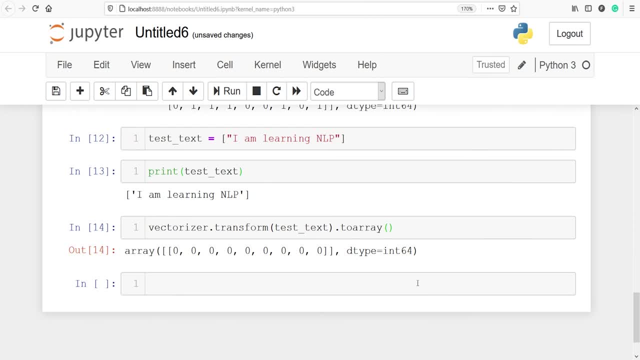 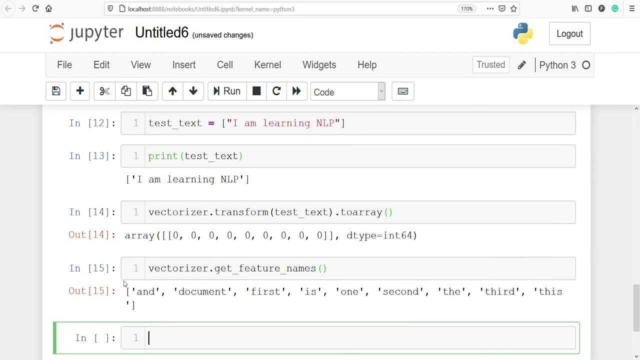 very similar. I will paste this here. and this is the feature name. if you compare the expression with the feature name, do you see the i is present in the feature name. we got 0 here. is am present. am is also not present. we got 0 here. 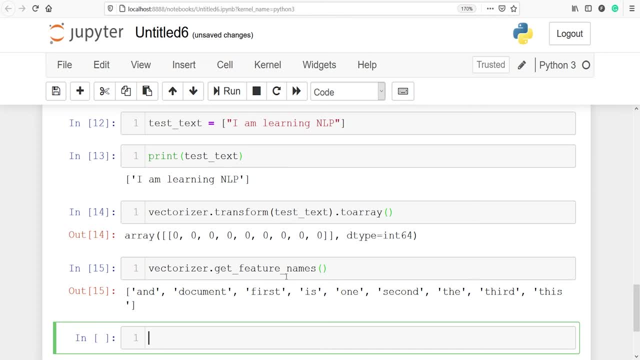 Learning. learning is the present. learning is also not present. we got 0 here and MLP is present, And as is� p is also not present here. so we got zero here and rest. all these zeros are for to to make it, uh, nine words, because in our vocabulary we are having nine words: one, two, three, four, five, six. 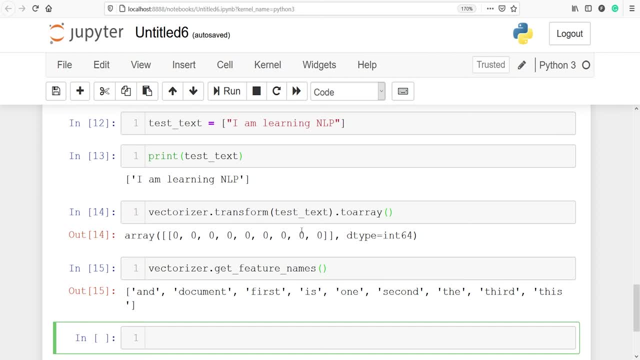 seven, eight and nine. that's why we got nine zero here. in actual, we are having only four zero one, two, three and four. but since our vocabulary has nine words, to fill those five words, we are putting five extra zero here and that is why we got nine zeros here. to overcome this problem, we can do one. 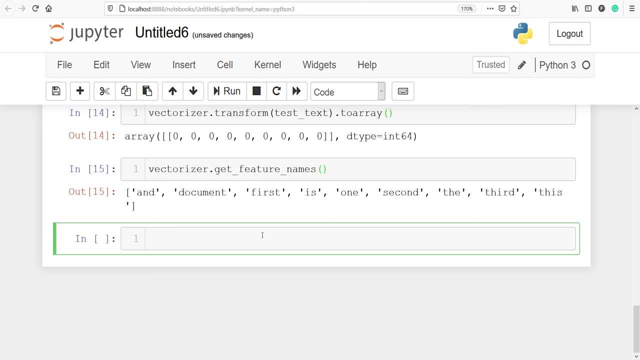 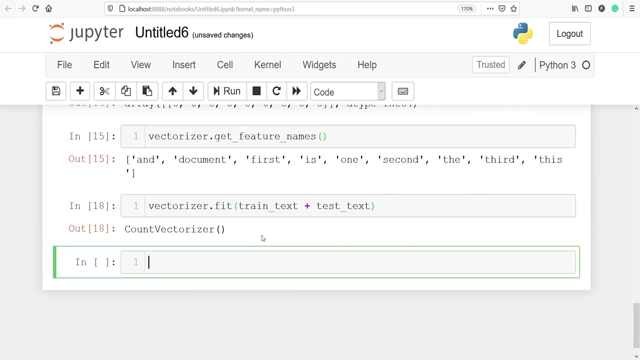 thing we can call the fit method. on the test data along with the train text, i'll call the object vectorizer and then i will call the property fit, and this time i am going to fit on both train and text. train text plus s underscore text. let's execute our code. let's look at the vocabulary to find the. 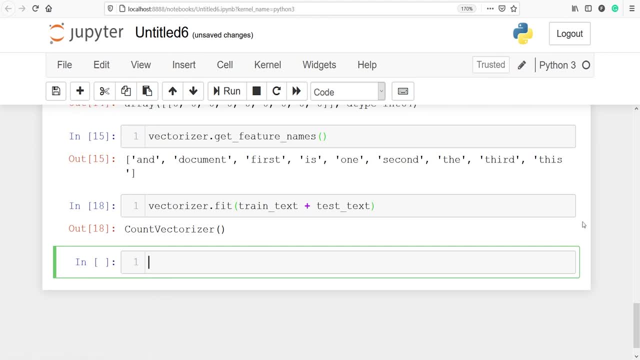 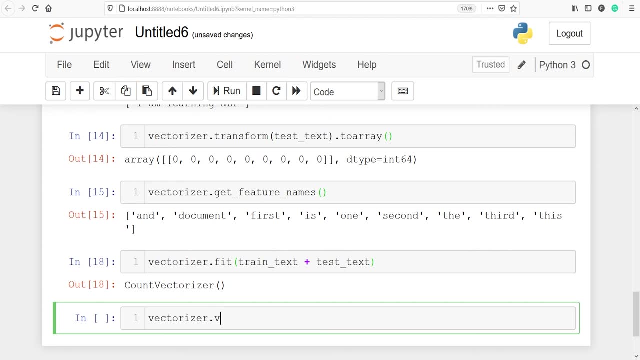 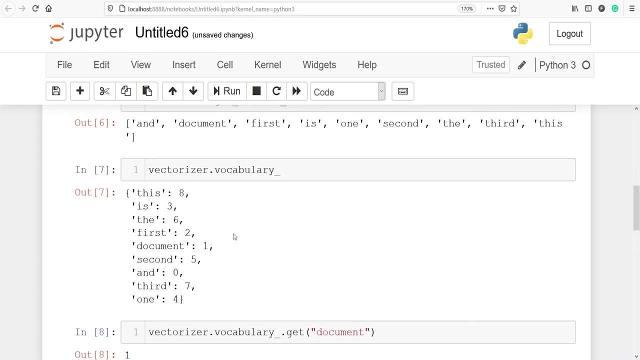 new words from the variable this test underscore text. i will call this object vectorizer and from this i will call the property vocabulary. and here we will see we have. here we have nine words, and so our vocabulary is z up from starting from zero to eight. let's execute our code and see. 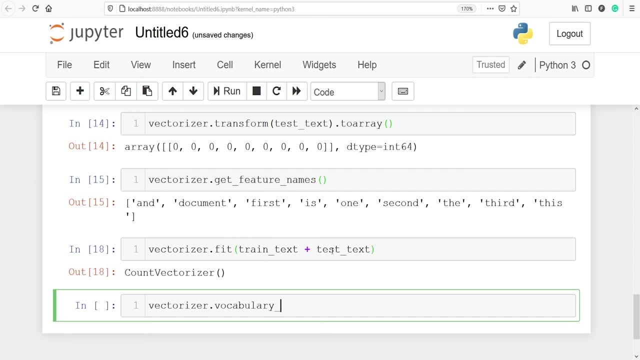 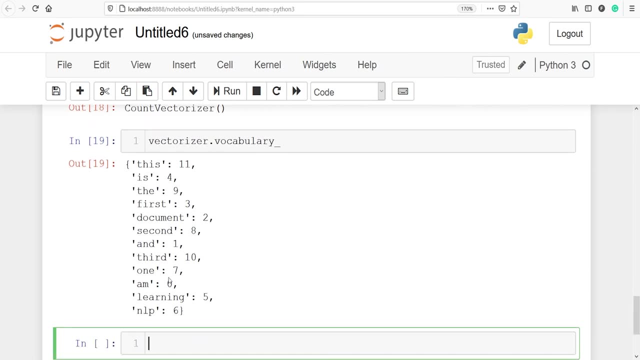 we will get new vocabulary because we have added this test underscore text variable. let's execute our code now. our vocabulary has increased, now we have new words such as nlp learning, and let's now transform our test underscore text. i'll call this vectorizer. then, from this transform. 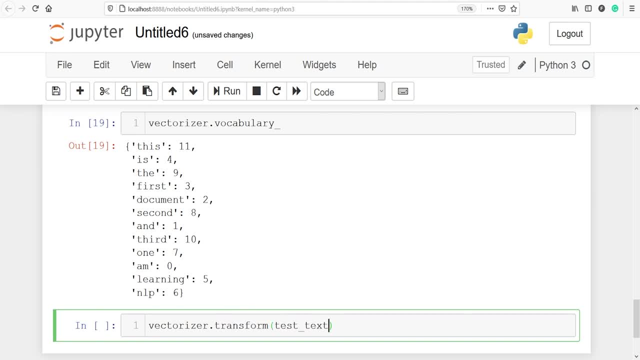 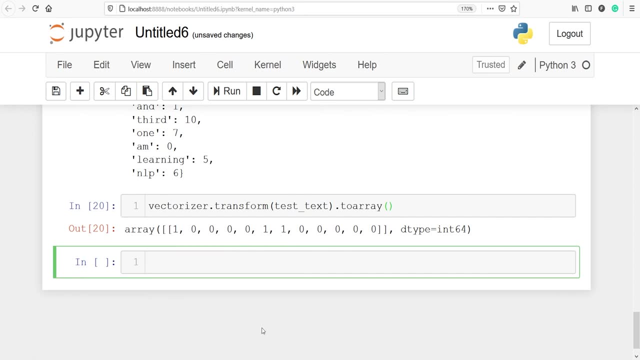 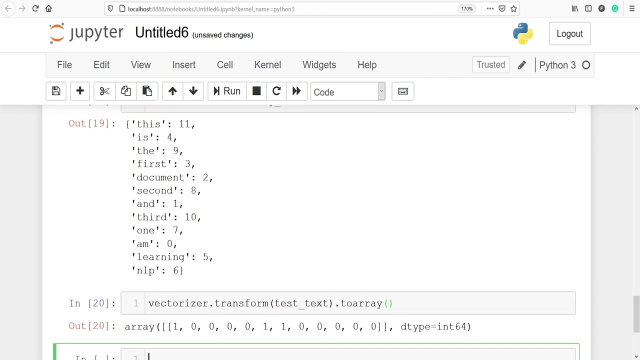 test underscore text and also convert it to array. let's execute our code in the output. you can see now we got 1 and 0. earlier we were getting only 0 here and we got 1. this video was about bag of words representation using count vectorizer. if you like my video, please subscribe to my channel. thank you for watching.